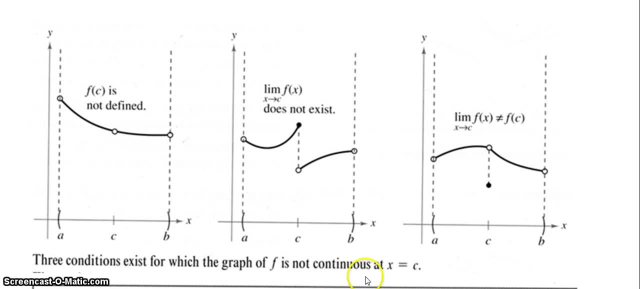 So there are three conditions that exist for which a graph f of f is not continuous at some value c, where c is just an x value. So here I have an open interval from a to b, and f of c is not defined, so there's just a hole there. 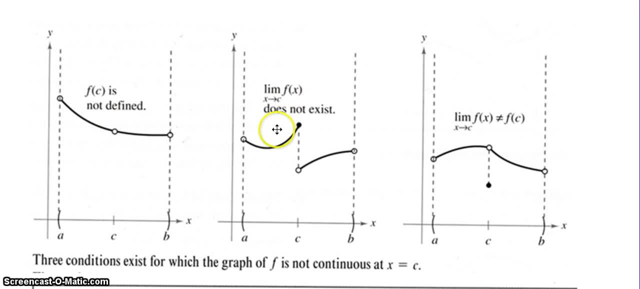 That's one way in which a function would not be continuous at c. Here the limit as x goes to c of f, of x does not exist. So if the limit doesn't exist, the function can't be continuous. And then the third scenario is: 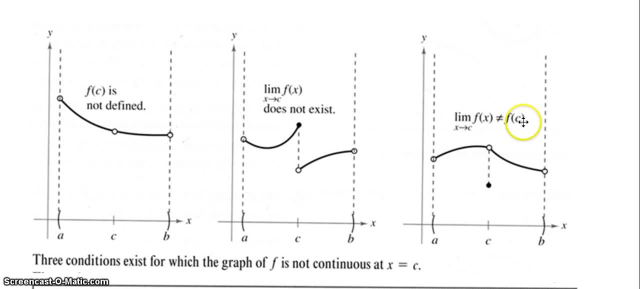 the limit as x goes to c of f of x does not exist. The limit as x goes to c of f of x does not exist. The limit exists but it's not the same as the function value at c. So that's the third scenario. 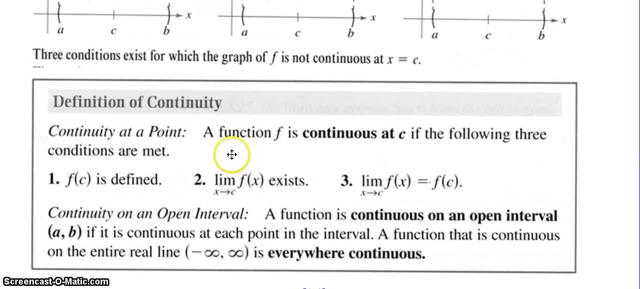 So what does this mean? So this is our definition for continuity at a point: a function, f, is continuous at c if the following three conditions are met: First, the function is defined at c. Second, the limit, as x goes to c of f, of x exists. 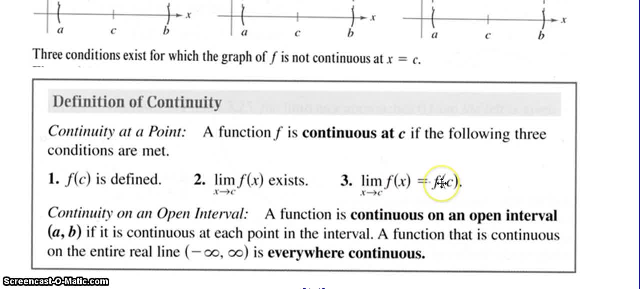 And third, the limit, as x goes to c of f, of x equals the function value. at that point, Again, as I said, this should make sense. It's kind of common sense in a way, That in order for something to be continuous it has to exist. 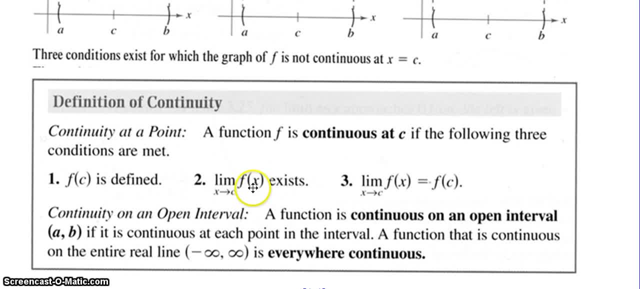 The limit has to exist, which that's just telling us, then from both sides it's approaching the same value, And the limit and the function have to have the same value. That should make sense. So continuity on an open interval. a function is continuous on an open interval a, b if it is continuous at every point in the interval. 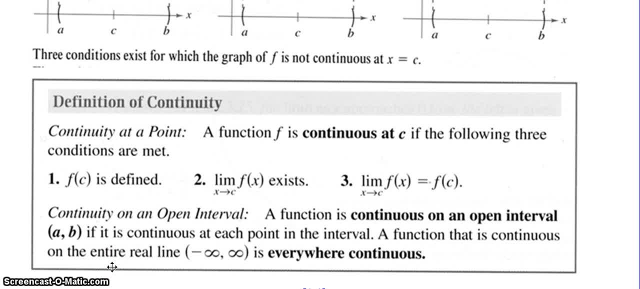 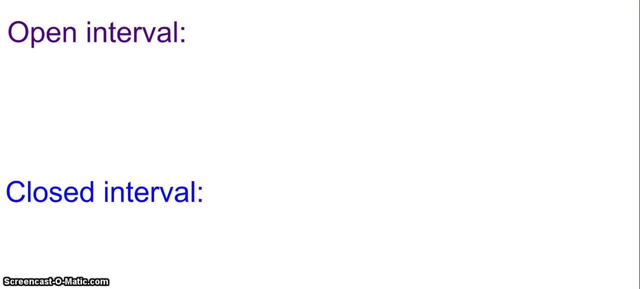 A function that is continuous on the entire real line. negative infinity to infinity Is what we call everywhere continuous. Okay, so real quick. let's make sure we really understand what it means to be an open interval versus a closed interval, Because these are words that come up a lot in these definitions. 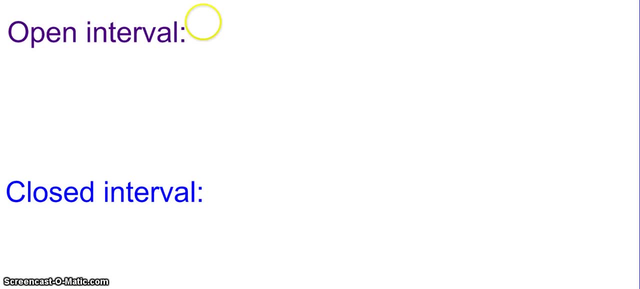 And again, they sound really fancy but they're not. So open interval is when we have our parentheses. Remember that. just doesn't that means we don't include the endpoints. So So, So, So, So So. 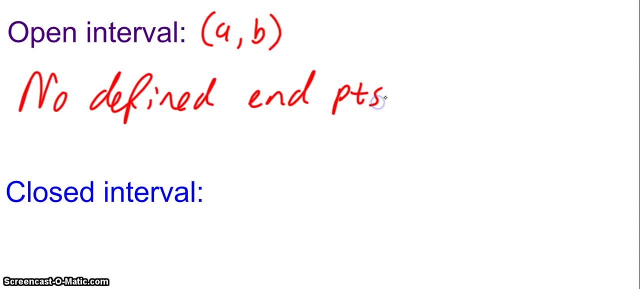 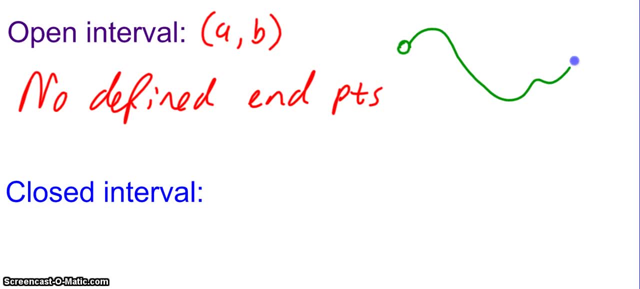 Open interval, something like this: So where this is our A and this is our B, So that would be an example of an open interval. Now I do want to point out an open interval could also be all real numbers. So negative infinity to infinity is an open interval because, remember, negative infinity and infinity are not actual values that we can get to. 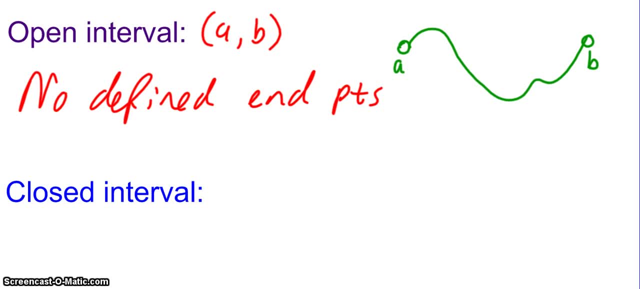 So then, a closed interval interval. well, that's when we have the brackets, So we're including the endpoints. So let's draw a picture. So that's my A now, and that's my B, That's a closed interval, So that's. 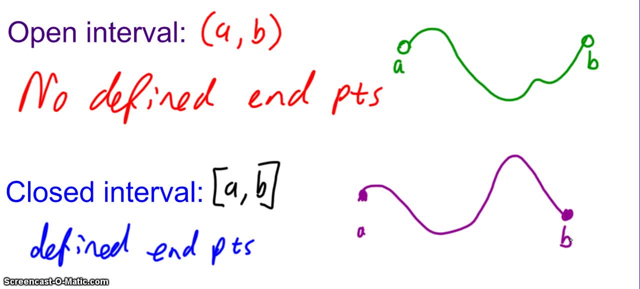 what we're talking about when we say open interval versus closed interval. Open interval- no defined endpoints- It doesn't mean that it's negative infinity to infinity. It could just be some segment, but we're just not including the endpoints, Or it could be negative infinity. 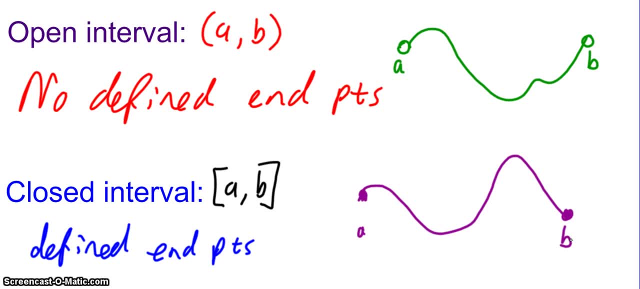 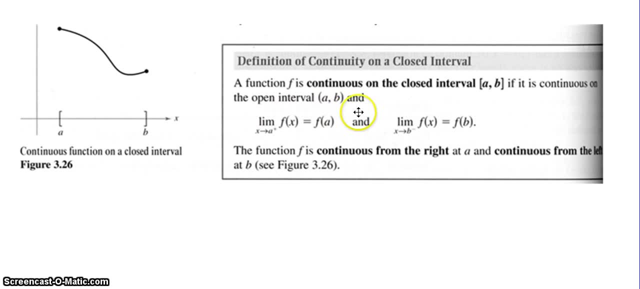 to infinity, But closed interval. we have defined endpoints, All right. so the previous definition was continuity on an open interval. So a definition of continuity on a closed interval is a function f or, I'm sorry, a function f is continuous on a closed interval A B. if it is continuous on the open interval A B, Okay, so it has. 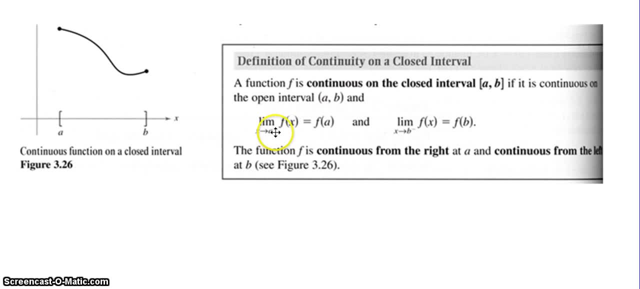 to meet that definition. And the limit as x goes to A from the right of the function is the function value at A, And the limit as x goes to B from the left of the function is the value of the function at B. So the function f is continuous on the open interval. 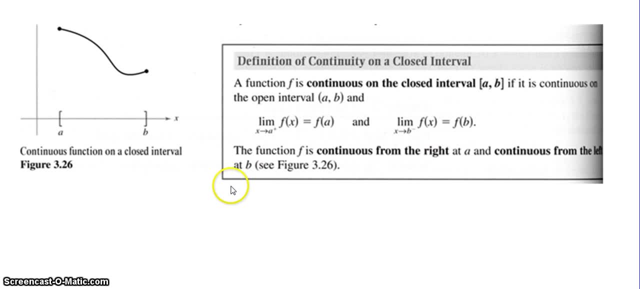 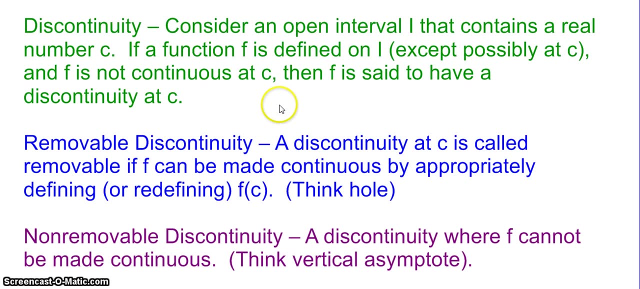 Continuous from the right at A and continuous from the left at B. That's our definition of continuity on a closed interval. So discontinuity: Consider an open interval, I that contains a real number, C. if a function f is defined on I, except possibly at C and f is not continuous. 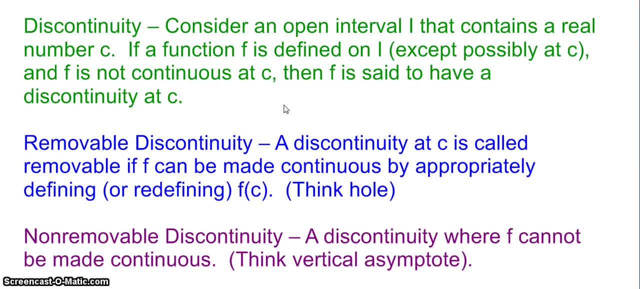 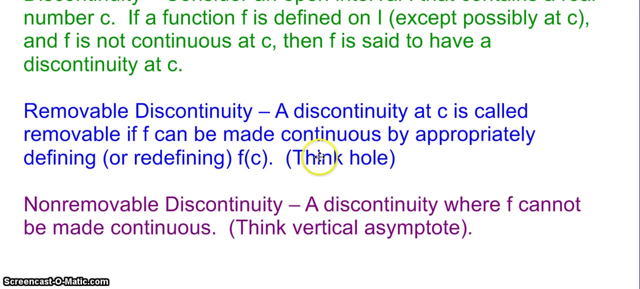 at C, then f is said to have a discontinuity at C. So if it's not continuous then it has a discontinuity Removable discontinuity is a discontinuity at C is called removable if f can be made Continuous by appropriately defining or redefining f of C. So, like I said before, think about. 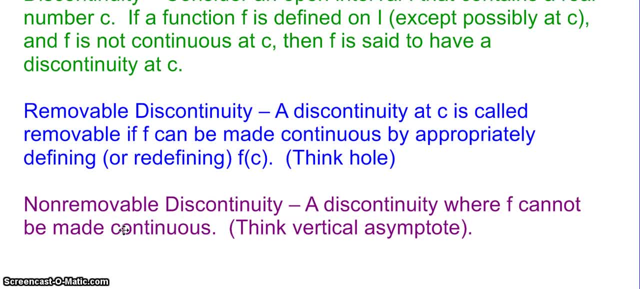 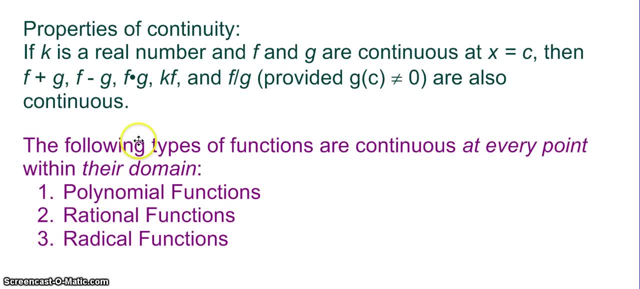 a whole Non-removable discontinuity is a discontinuity where f cannot be made continuous. So think about an asymptote or a jump. So properties of continuity. if k is a real number and f and g are continuous at x equals C, then f plus g, f minus g, f times g, k times f and f over g, assuming that g of 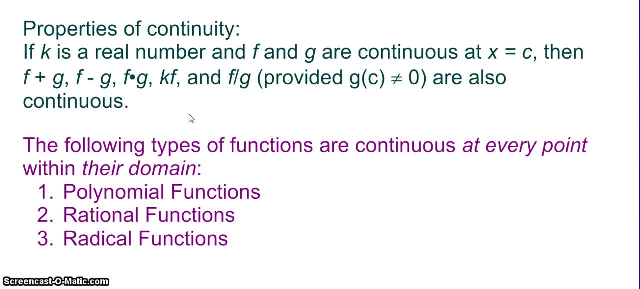 C is not zero- are also continuous. So that's just saying that if we add, subtract, multiply, divide, multiply by a scalar any two continuous functions at some value, then that result will also be continuous. The following types of functions are continuous at every point within their domain. We've 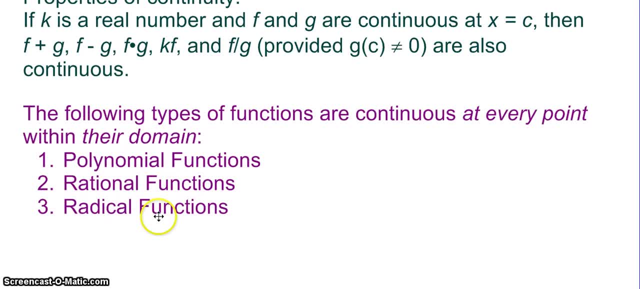 actually talked about this earlier in first semester when we talked about polynomials, rational functions and radical functions. So these functions are continuous everywhere within their domain. It's very important that we understand that this is within their domain, because rational functions and radical functions do not have a domain of all real numbers. 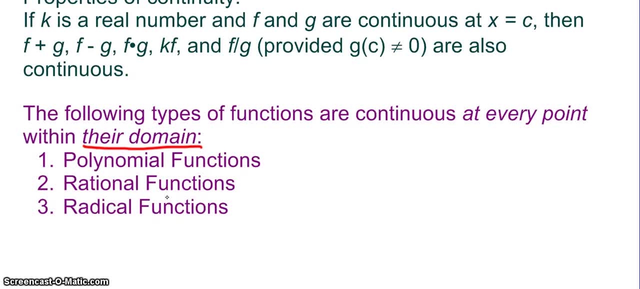 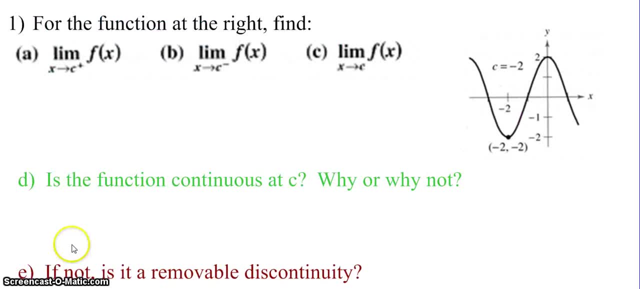 necessarily. They can, but they don't have to, But they are still continuous everywhere. within their domain- Polynomial functions- they have a domain of all real numbers. Okay, so let's try some examples. So for the function at the right, I want you to find: 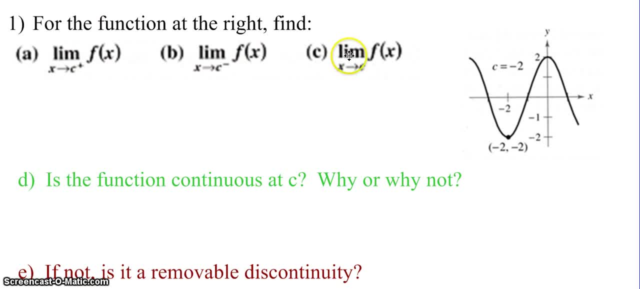 the limit as x goes to C from the right, the limit as x goes to C from the left and the limit as x goes to C, Then determine if the function is continuous at C, state why or why not, And if not, is it a real number? 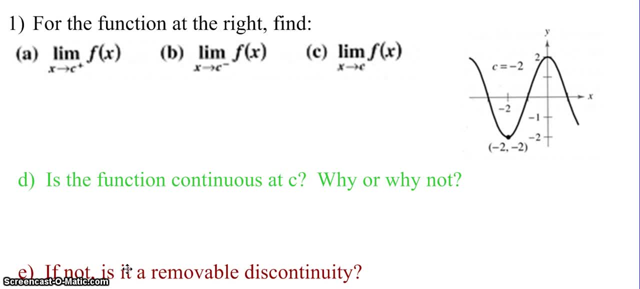 Is it a removable discontinuity? Pause the video. do that unpause and be ready to check. Alright, so hopefully you figured out that the limit as x goes to C from the right is negative 2.. The limit as x goes to C from the left is also negative 2.. 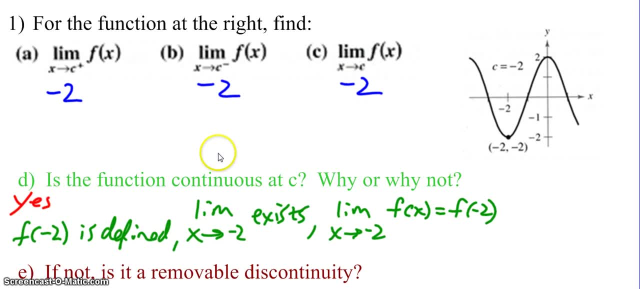 Therefore the limit as x goes to C from the left and the right is negative 2.. So the function is continuous at x equals C and our reason is because it meets our three questions. Qualifications f of negative 2 is defined. the limit as x goes to negative 2 exists. 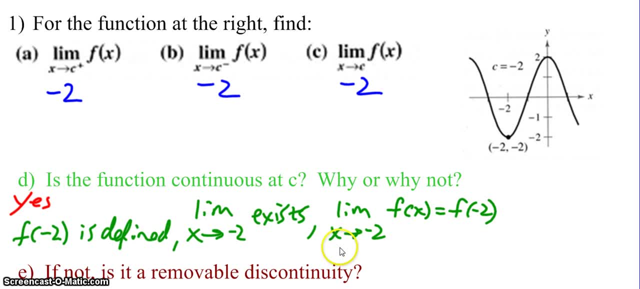 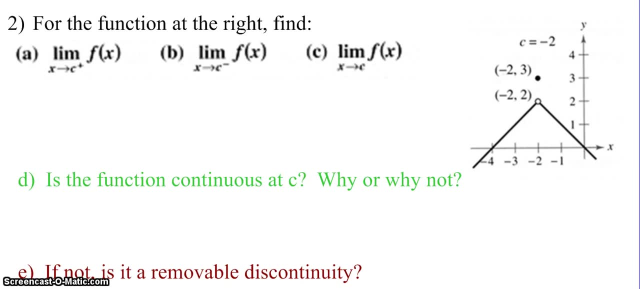 and the limit as x goes to negative, 2 of f of x equals f of negative 2.. So we don't have to worry about e, because it's not applicable here. Alright, I want you to try this one Same idea: pause the video, unpause and be ready to check. 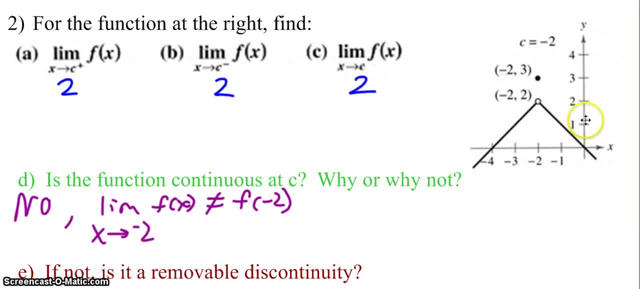 Alright. so again, the limit as x goes to C from the right or as x goes to negative 2 from the right is 2. in this case, The limit as x goes to negative 2 from the left is also 2, therefore the limit as x goes. 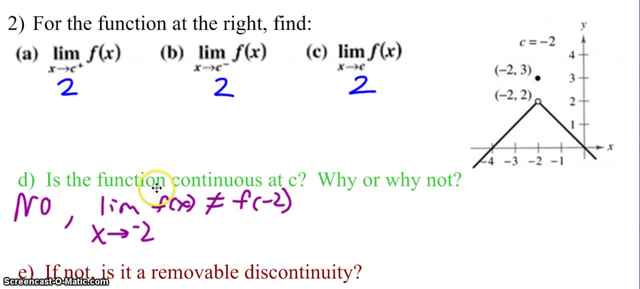 to negative, 2 from the left and the right is 2.. Is the function continuous, though? No, it is not. Again, this should be obvious, like I see that. But why is it not? Well, it fails. the third requirement. 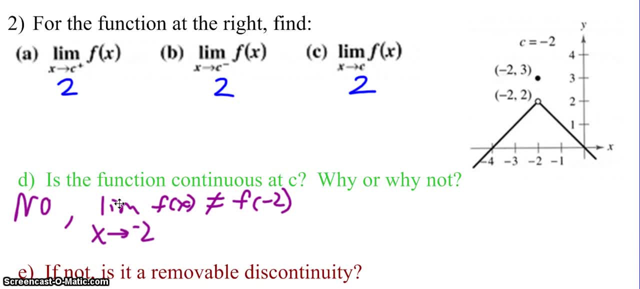 So it did meet the first and second requirement. where f of negative 2 was defined, the limit does exist, but the limit as x goes to negative 2 of f of x does not equal f of negative 2.. Okay, Is it a removable discontinuity? 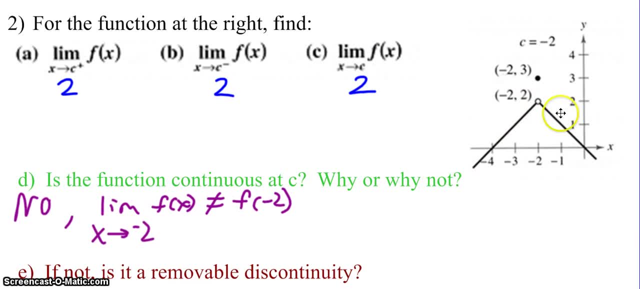 Yes, it is, Because this is a whole. we could come up with a different function that is exactly the same everywhere, except for at the discontinuity, and then would therefore be continuous. Next, one same thing: pause the video, unpause and be ready to check. 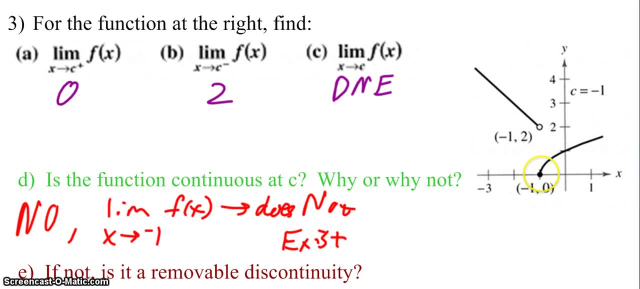 Okay, so here the limit as x goes to negative 1 from the right is 0,. the limit as x goes to negative 1 from the left is 2,. therefore, the limit as x goes to negative 1 does not exist from the left and the right. 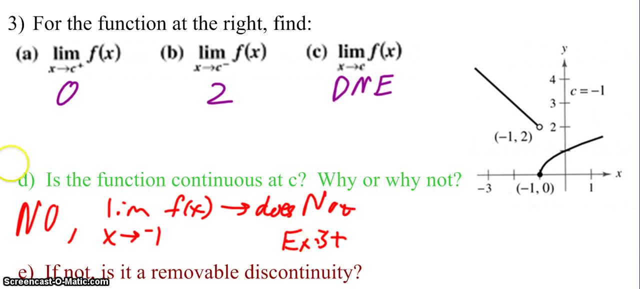 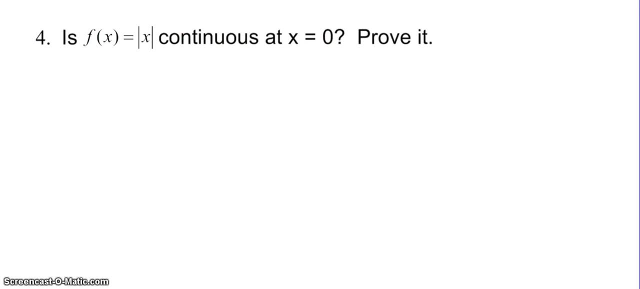 So the function is not continuous because the limit does not exist and it is not a removable discontinuity. Alright, so I want you to prove that f of x equals absolute value of x is continuous at x equals 0.. By prove I really mean just show. it's not really a proof. 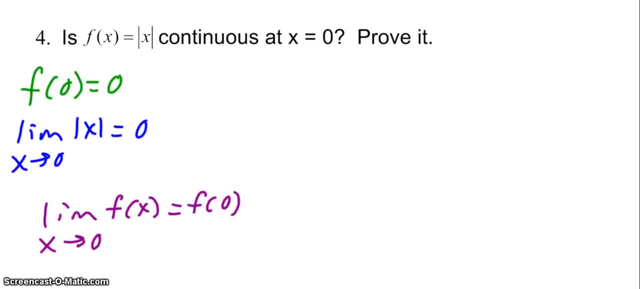 Pause the video. unpause and be ready. show Alright. so for a question like this, really, all you're doing is you're just showing that all of our three requirements are met. So the function exists, The limit exists and the limit equals the function value at that x value of 0 in this. 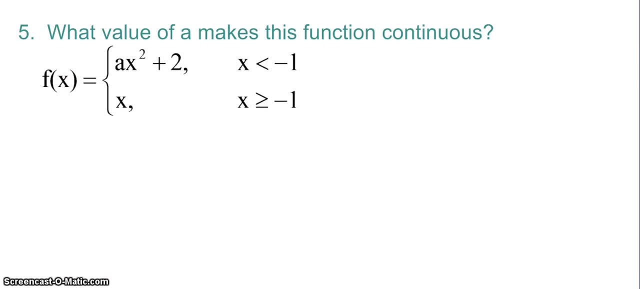 case. Alright, I want you to try this one now. Find what value of a will make this function continuous. So pause the video, do that unpause and be ready to check and think about the requirements. Alright, so the first thing I notice is that each piece of the function is continuous. 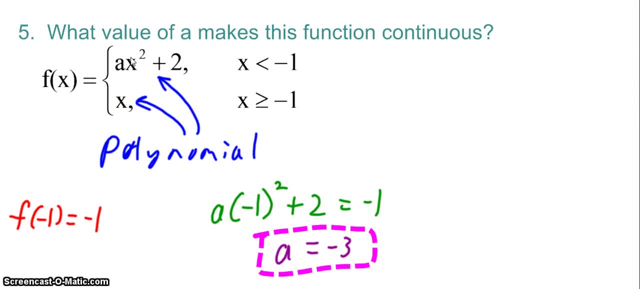 Each piece of this piecewise function is a polynomial And therefore remember that a polynomial is continuous everywhere. So the only possible point of discontinuity of the piecewise function is where I jump from one piece to the other, which happens at negative 1.. 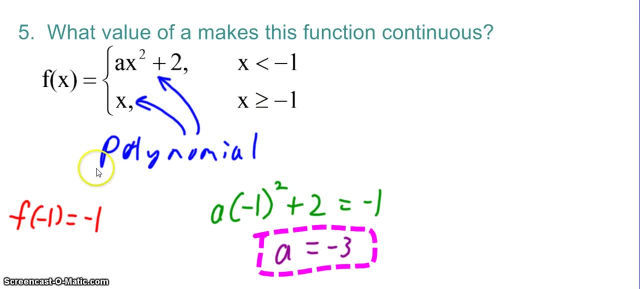 And so all I need to do is I need to figure out, okay, what is the current y value when x is negative 1.. So I plug in negative 1 to the piece that includes negative 1, which gives me negative 1.. 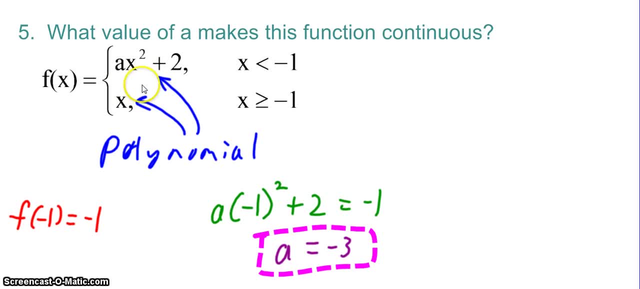 And then I need to make this other piece have that same value. So if that happens then the limit will exist. the limit will equal the value. so I'll meet my requirements. So I do: a times negative: 1 squared plus 2 equals negative 1.. 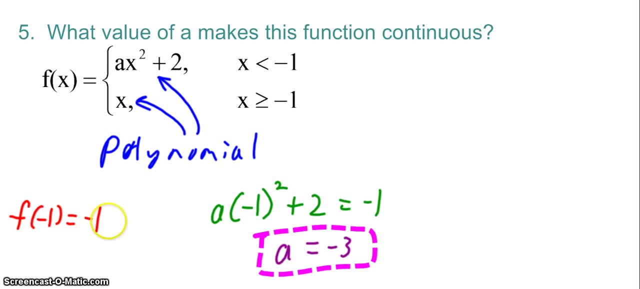 And again, this negative 1 here is because that's what the function equaled. This negative 1 is because that's what I'm plugging in. So when I solve that, I get a equals negative 3.. So if a is negative 3.. 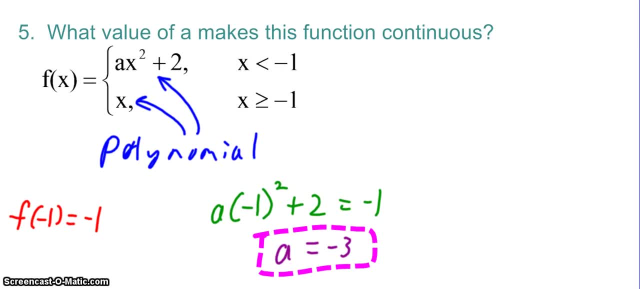 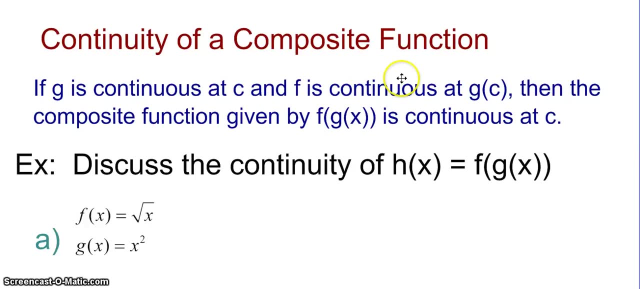 This piecewise function will be continuous. Alright. so now let's look at the continuity of a composite function. So if g is continuous at c and f is continuous at g, then the composite function given by f of g is continuous at c. 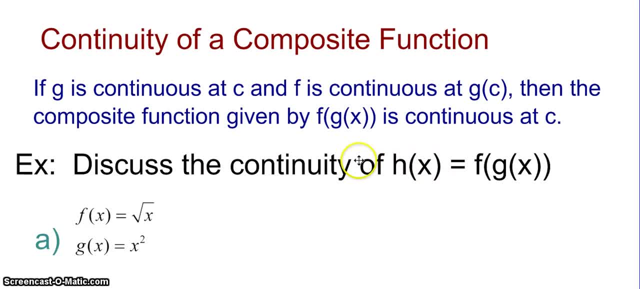 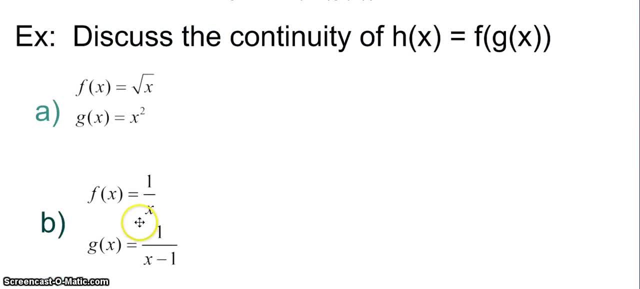 Okay. so now we want to think about the continuity of the following two functions, or the following functions: So if f of x is the square root of x and g of x is x squared, and then we also want to think about what if f of x is 1 over x and g of x is 1 over the square. 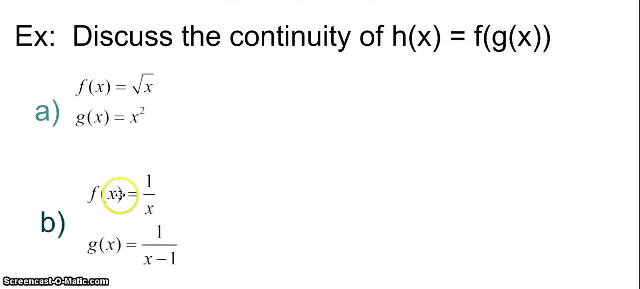 So, instead of t of x, what if f of x was 1 over x, the square root of x? i'm sorry, fx is 1 over x and g of x is 1 over x minus 1. i apologize, so i want you to pause the video and think about what the resulting continuities are going to be for these. 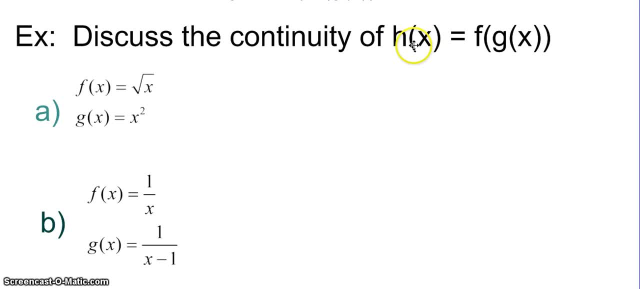 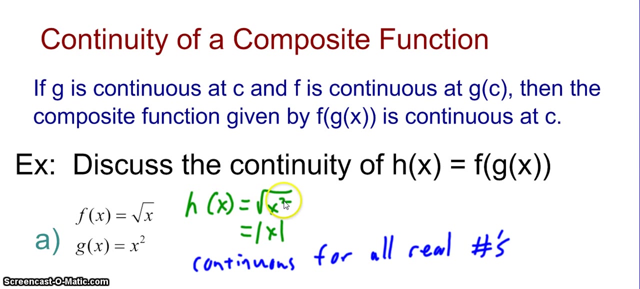 for the compositions for h of x. so that's what you're trying to figure out: what is the continuity of h of x? pause the video. unpause when you're ready to discuss, because that's what we're doing is discussing. okay, so the first one, h of x, equals the square root of x, squared which, remember that. 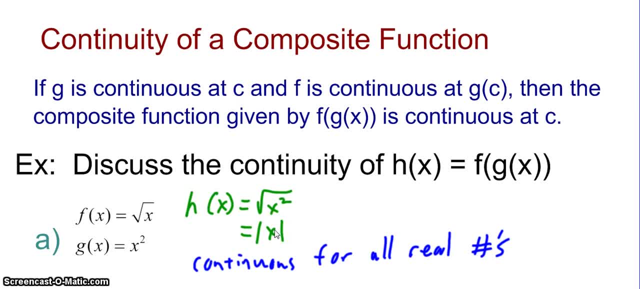 simplifies, actually by definition, to the absolute value of x, which is something that is continuous everywhere. so h of x is continuous for all real numbers. now if i look at this definition up here, i know that g of x is a polynomial which is continuous everywhere. so g of x is continuous. 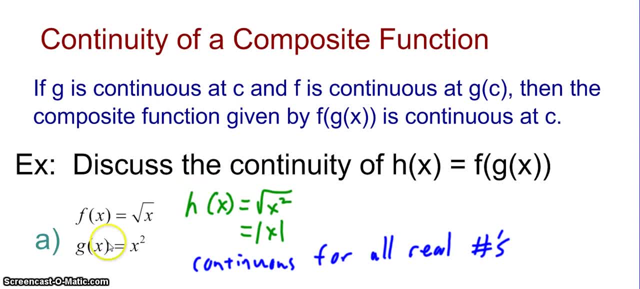 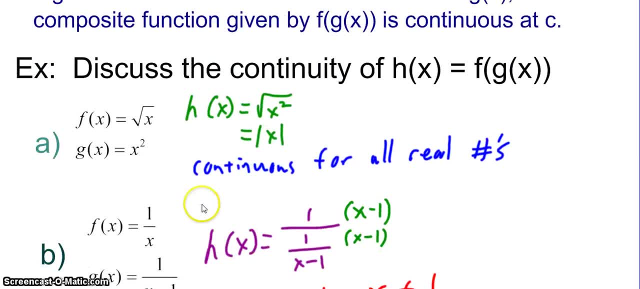 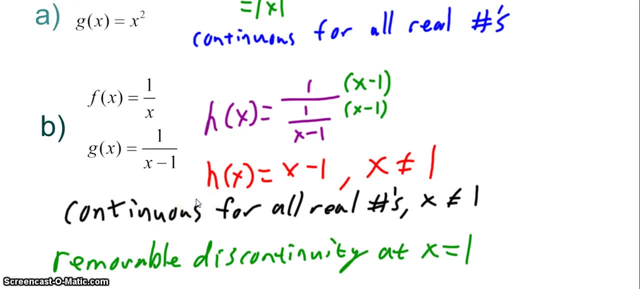 at x equals c and f then is continuous at x equals c, continuous at g of c. so this means my definition is continuous for all real numbers down here it's a little trickier and this remember really what we're talking about. so we're defining continuity really formally. um, really it's just talking about the domain. 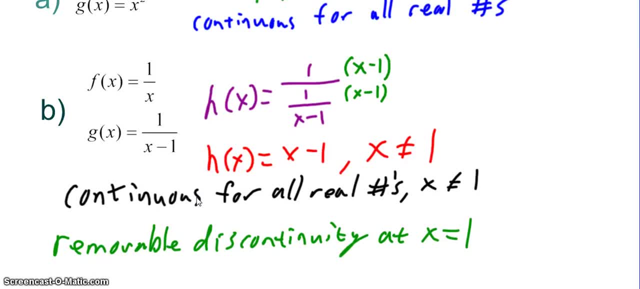 of a function in some ways. i mean, there's not exactly, but there's a lot to do with domain. so if i compose f of g of x, which is h of x, i do 1 over 1 over x minus 1. i don't like the. 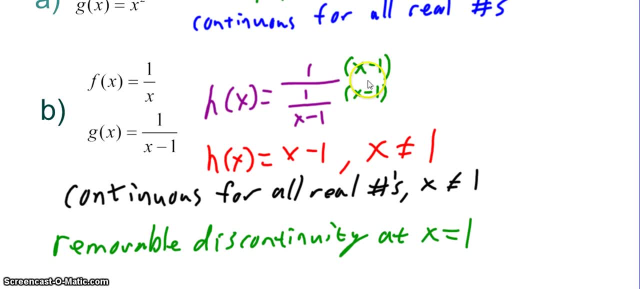 division of fractions. so i multiply the numerator and denominator by the reciprocal of the numerator, which is just x minus 1, and i end up with the h of x is just the function x minus 1. but remember when we did composition of functions back in first semester and we talked about how 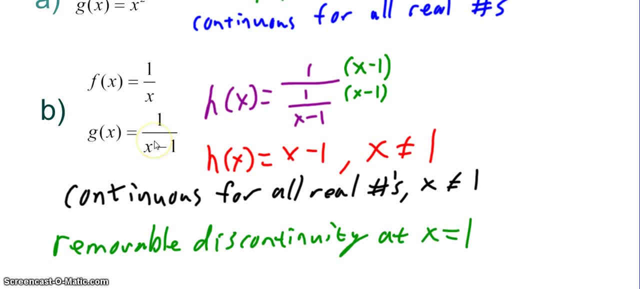 does the domain work? well, the domain is restricted by the function that we plug in. so the restricting on the function of g of X is that X cannot equal 1. so therefore, although H of X simplified to a polynomial, it still can't equal 1. so this is continuous for. 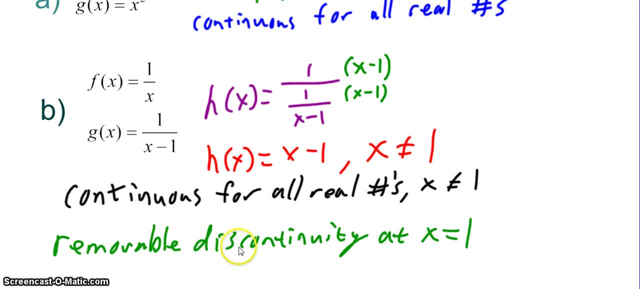 all real numbers except for at X equals 1, and I also know this is a removable discontinuity because of the fact that this is a polynomial, so I know I can write this polynomial where it does exist: at X equals 1. so that's what makes 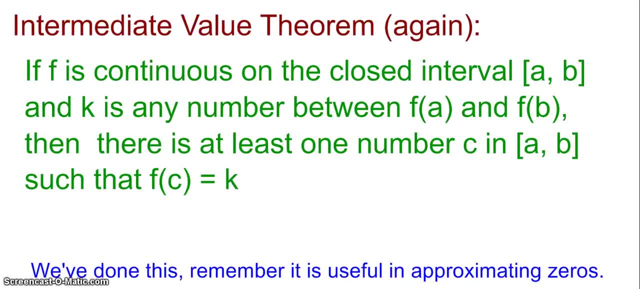 it removable, alright. last thing we're going to talk about today is the intermediate value theorem. we have talked about this before. all it says is that if f is continuous, so now we're bringing it back up because it has to be continuity on a closed interval- a to B and K is any number between f of a and F. 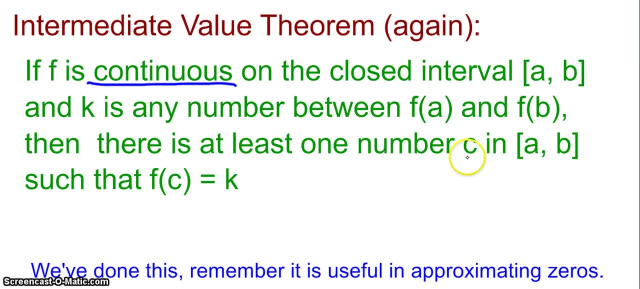 of B, then there is at least one number- see in a to b, such that f of C is K. we've done this before. we've used it for approximating zeros. you can use it it to approximate any number. but really the usefulness that we've seen before is: